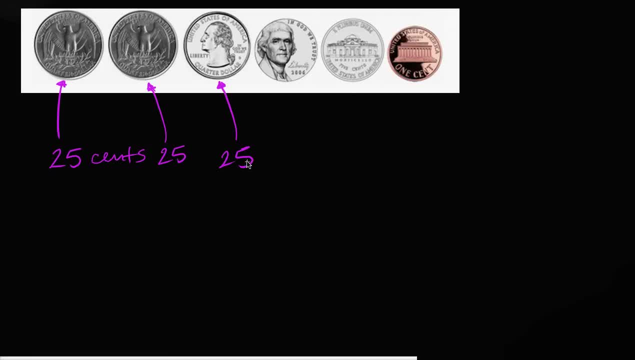 Well, it's going to be 25 plus 25,, which is 50, plus 25,, which is going to be 75. So these three quarters are going to be 75,, 75 cents And, remember, 100 cents. make a dollar. 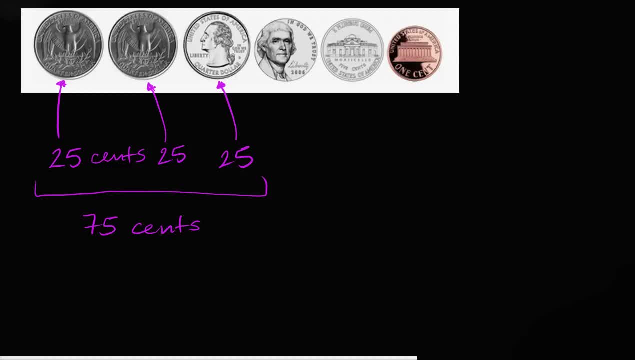 so this is still less than one dollar. But we're not done yet. We have this nickel- This is a nickel right over here That represents five cents. And then we have another nickel here. It looks different, but it's just the other side. 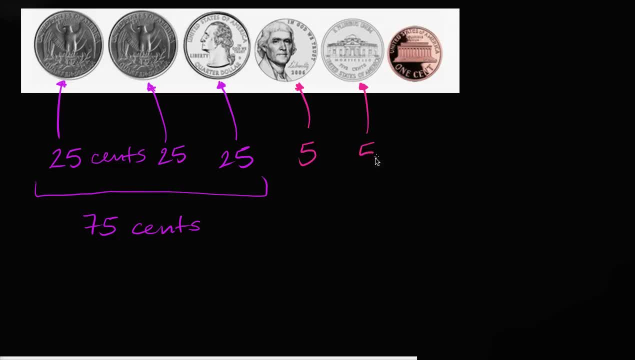 This is the head side, This is the tail side, So this is also another five cents, And so these two nickels, if you add them together, they are going to represent 10, 10 cents, And then, finally, you have a penny. 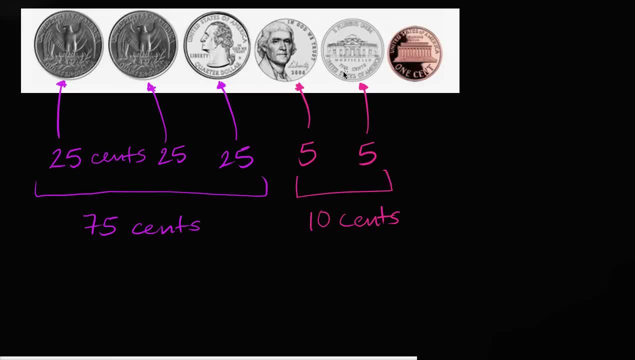 And a penny- and it even says it right over here- is one cent. In fact, they all say it here: This is five cents, This is one cent. So this right over here is going to be one cent. So what is 75 plus 10 plus 1?? 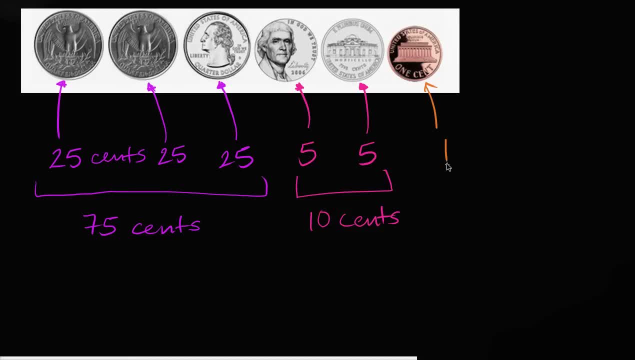 Well, 75 plus 10 is 85, plus 1 is 86. So this is equal to 86 cents. And if it felt a little bit too fast to count up 25,, 50,, 75 in your head, you could do this. 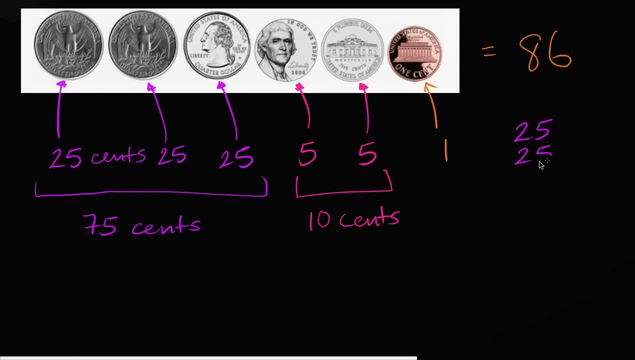 You could also add them up: 25,, 25,, 25, plus 5, plus 5, and another 5, plus 1, plus 1.. You could add them up this way, And then what would you get? 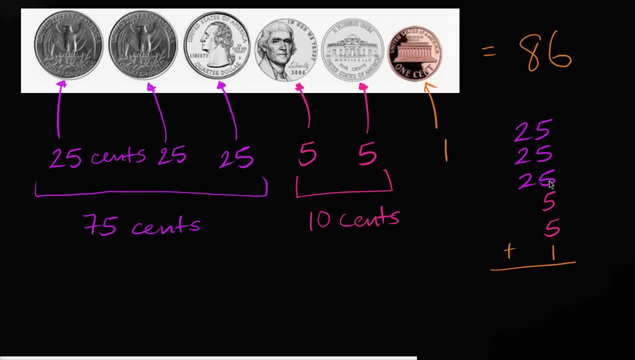 5 plus 5 is 10, plus 5 is 15, plus 5 is 20, plus 5 is 25, plus 1 is 26.. So that's two 10s and one 6.. Put the two 10s up here. 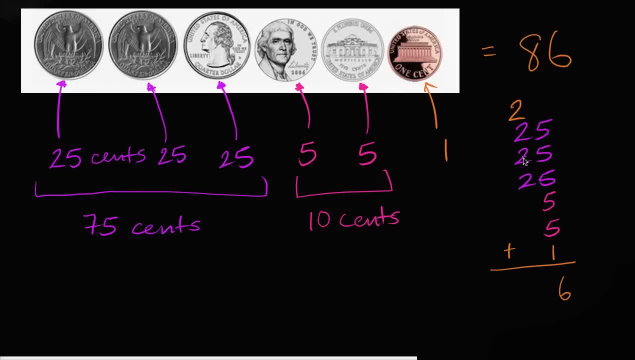 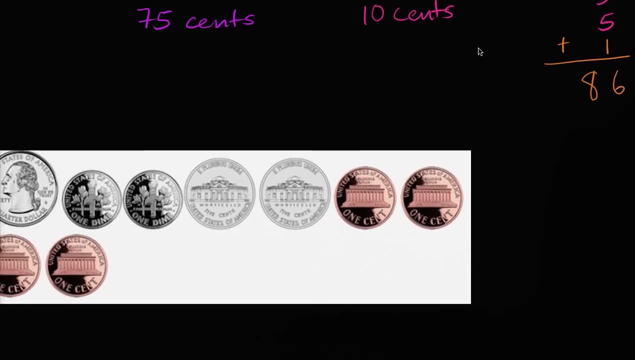 2 plus 2 is 4,, 4 plus 2 is 6,, 6 plus 2 is 8.. So you could get 86 cents either way. Let's do one that has even more coins in it. So here we go. 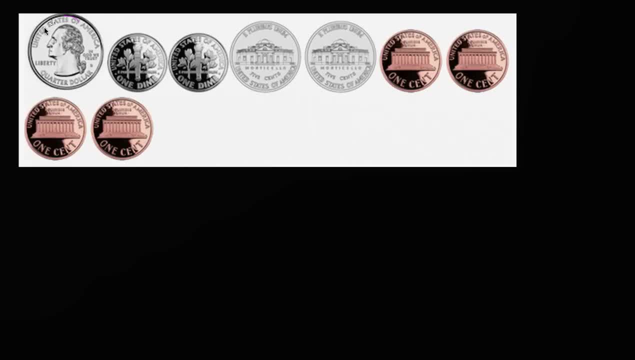 We have. so what is it? What's going on here? This right over here is a quarter That's going to be 25 cents, And then we have one that we didn't see in the previous example. We have two dimes. 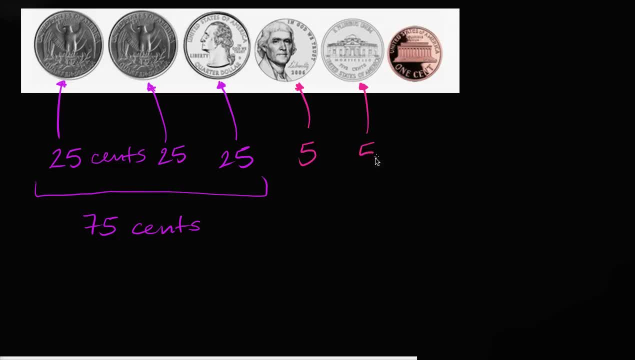 This is the head side, This is the tail side, So this is also another five cents, And so these two nickels, if you add them together, they are going to represent 10, 10 cents, And then, finally, you have a penny. 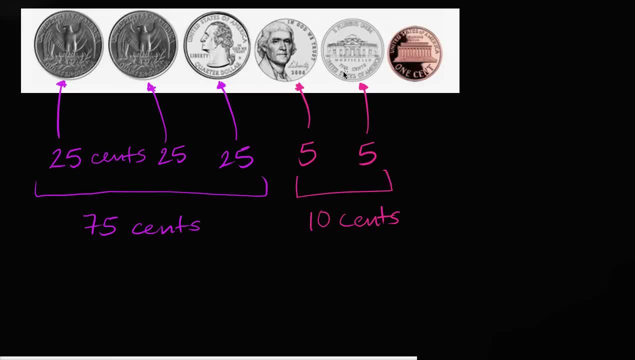 And a penny- and it even says it right over here- is one cent. In fact, they all say it here: This is five cents, This is one cent. So this right over here is going to be one cent. So what is 75 plus 10 plus 1?? 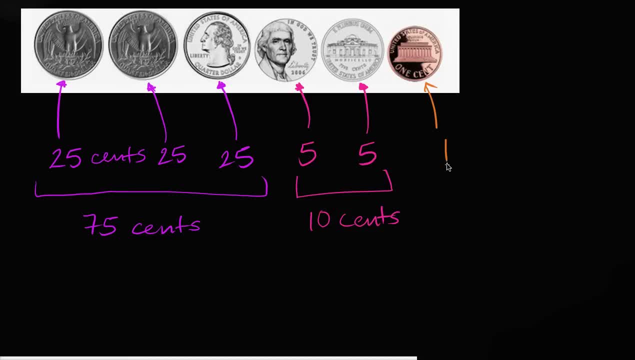 Well, 75 plus 10 is 85, plus 1 is 86. So this is equal to 86 cents. And if it felt a little bit too fast to count up 25,, 50,, 75 in your head, you could do this. 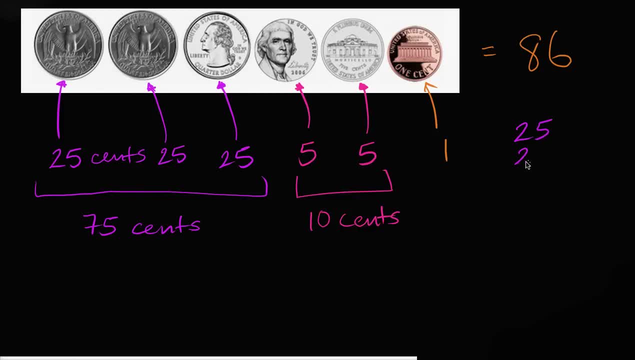 You could do this. You could also add them up: 25,, 25,, 25, plus 5, plus 5, and another 5, plus 1, plus 1.. You could add them up this way, And then what would you get? 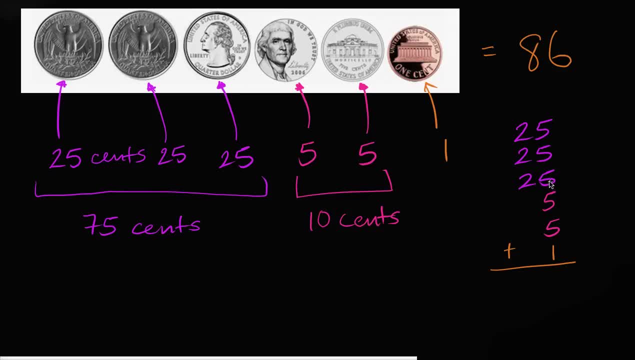 5 plus 5 is 10, plus 5 is 15, plus 5 is 20, plus 5 is 25, plus 1 is 26.. So that's two 10s and one 6.. Put the two 10s up here. 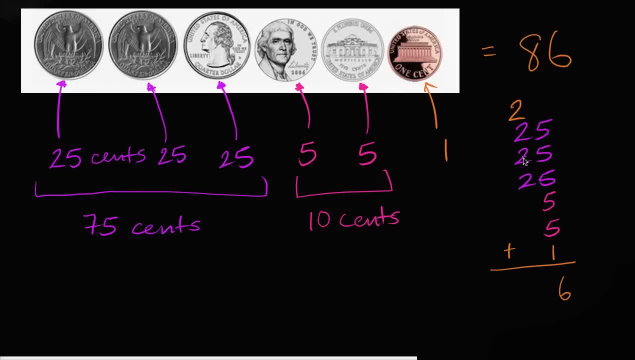 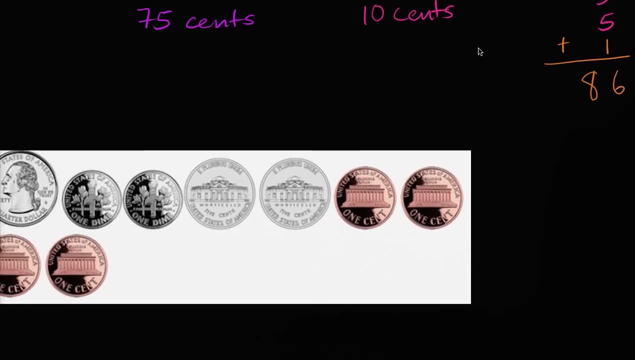 2 plus 2 is 4,, 4 plus 2 is 6,, 6 plus 2 is 8.. So you could get 86 cents either way. Let's do one that has even more coins in it. So here we go. 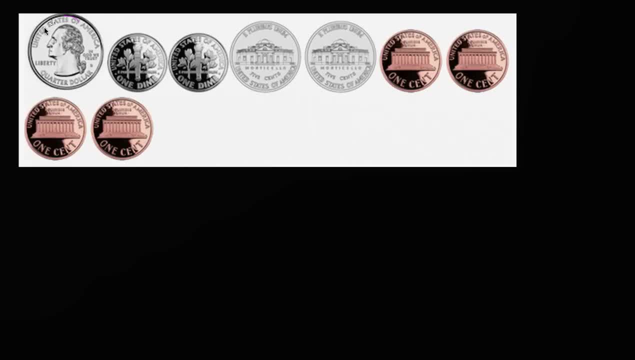 We have. so what is it? What's going on here? This right over here is a quarter That's going to be 25 cents, And then we have one that we didn't see in the previous example. We have two dimes. 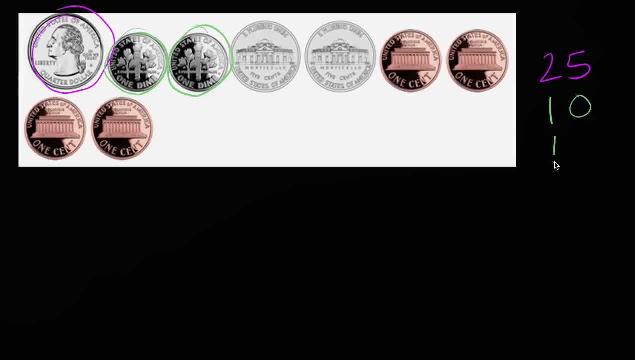 A dime represents 10 cents. So we have two dimes, Or we could have those- each represent 10 cents. Then we have two nickels. We've already seen those each represent 5 cents, So 5 and 5.. And then we have four pennies. 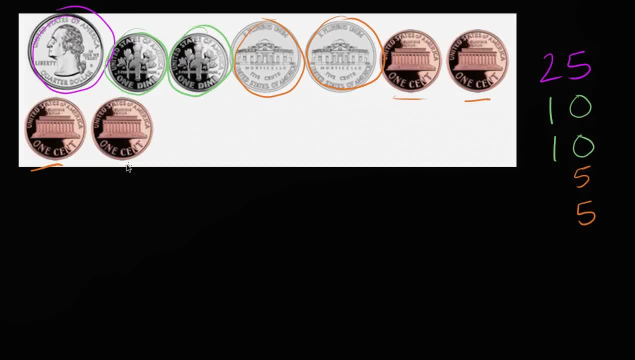 1, 1,, 2,, 3,, 4.. Now we could put each penny separately, like that. Or we could say: look, four pennies. each of them represent 1 cent, So that's going to be 4 cents.